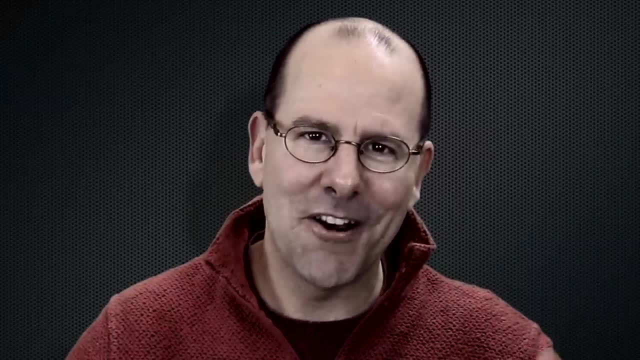 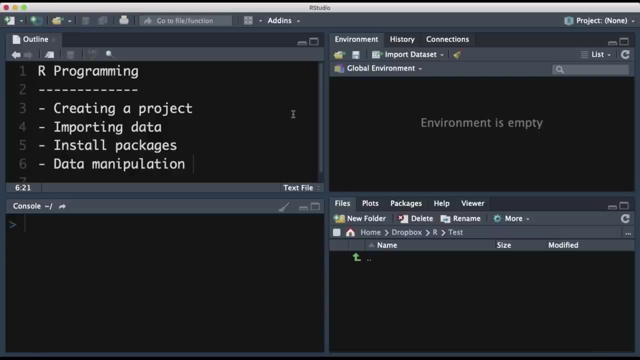 place On this YouTube channel. we're creating R programming videos on everything Right. we're looking at R studio At this point. you've installed R. you've installed R studio. If you're not familiar with this environment, there's these four quadrants. I've got a video that. 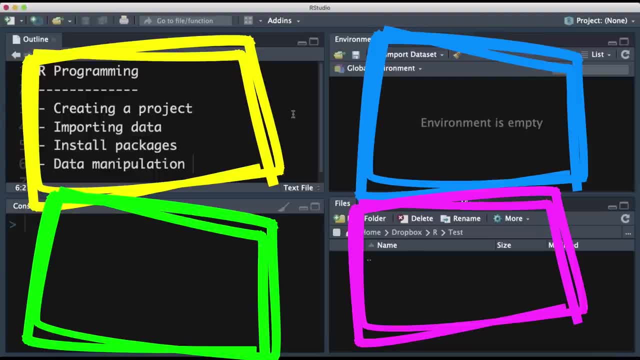 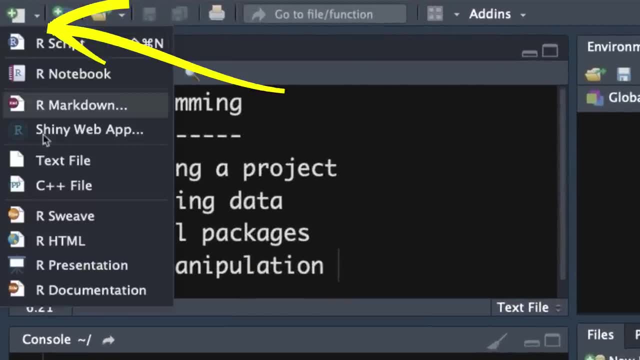 goes through that and introduces you to this environment. So have a look at that video. I'm not going to go through it right now. You're wanting to get going right. So at the top on the left you've got a little pull down menu and you've got some options. 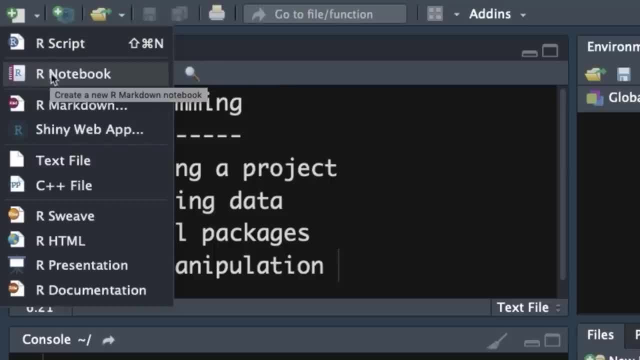 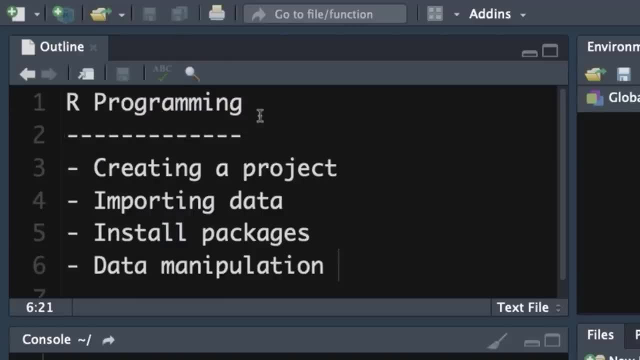 things you can start. There's an R script, R notebook. We're going to go through each of these in detail in future videos. I'm going to suggest ignore these for now. right Start off by starting a project. So just to the left you're going to see create a project button. 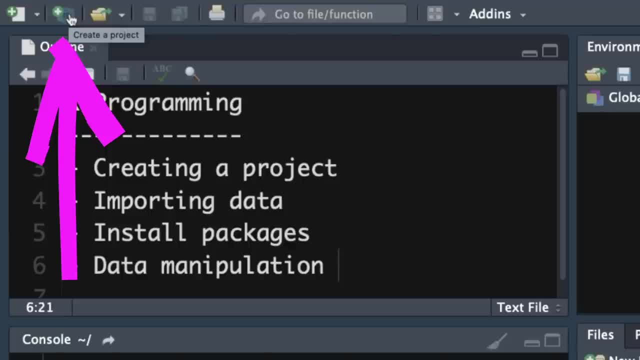 And the reason is: if you write your script in the context of a project that you've started, R will know where to look for your data, where to put all of your data, where to put all of your data. where to put all of your data? 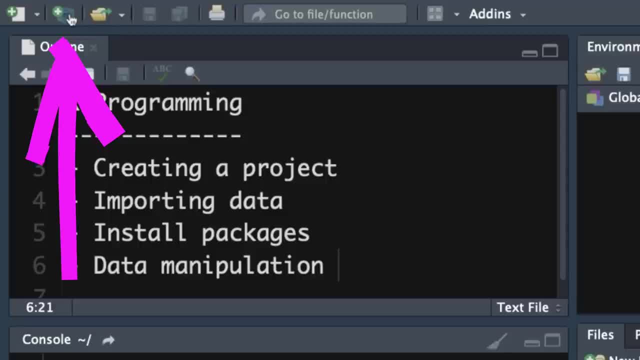 Your output, your graphics, et cetera, et cetera. It stores everything quite neatly in one place. It sets what we call your working directory, And that's quite a useful thing. You're going to find it more and more useful down the line. So my suggestion is right off the get go. 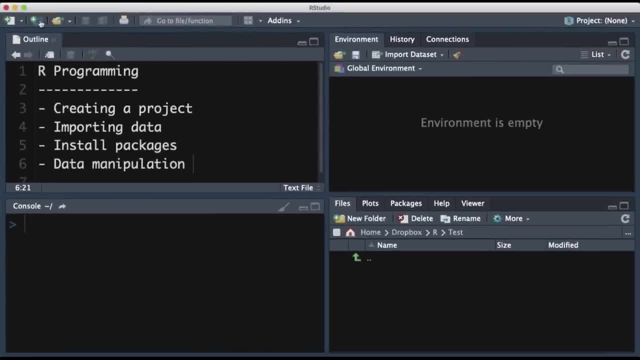 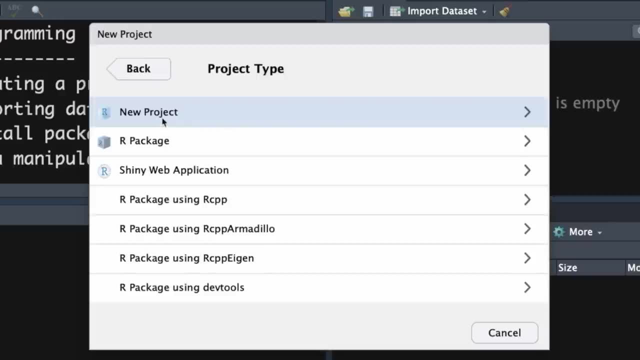 get into the habit of. when you're starting a project in R, click on the start a project button. You've got an option And I'm going to suggest create a new directory, a new project, give the project a name and I'm going to call it test. 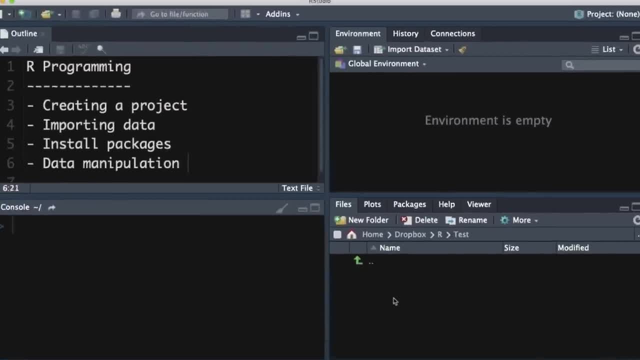 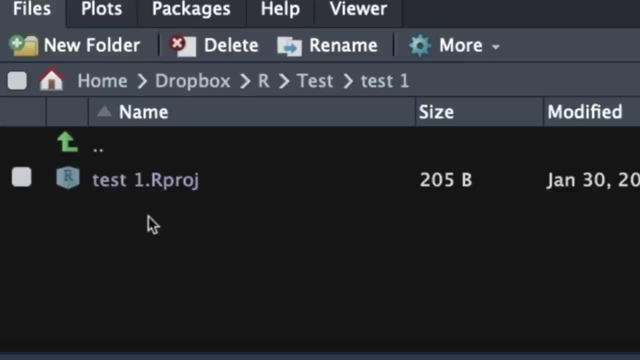 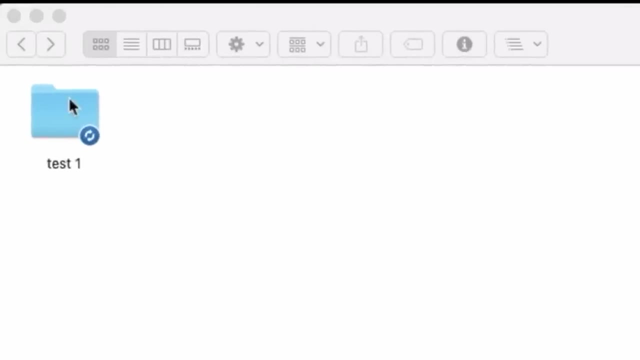 one like that and say: create project. Okay, so R has created a project. We can see the project down here at the bottom on the right, just so that you can see what's happening at the same time on my hard drive. If we have a look at my hard drive, R has created a folder called test one. Click on. 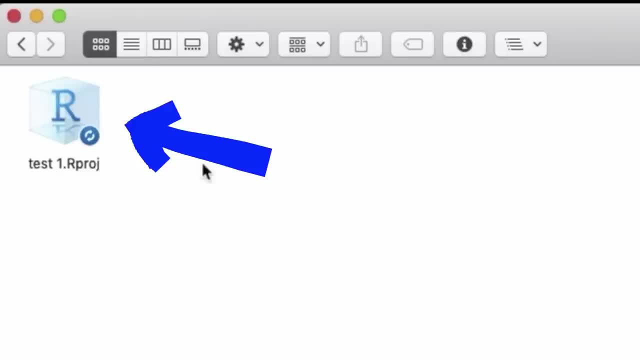 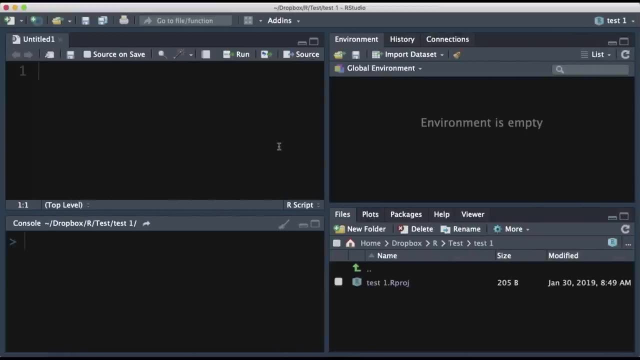 that folder and there we can see the little icon that represents the project. If R was closed and we went to this place on my hard drive, clicked on that icon, R would open up in that project and we would see all of the script and the data and the outputs from that project all in one place. It 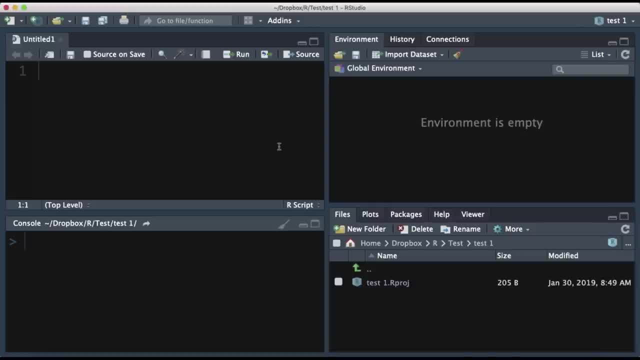 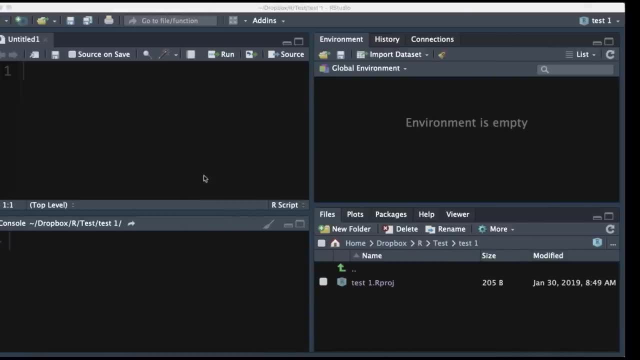 would be very neat, It would be lovely, It would be poetry. You're going to love it. Okay. so that's starting a project. Okay, so how do we get some data into R? Well, let's go back to our hard drive. 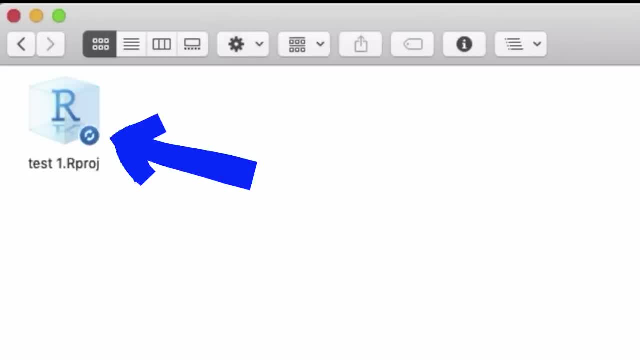 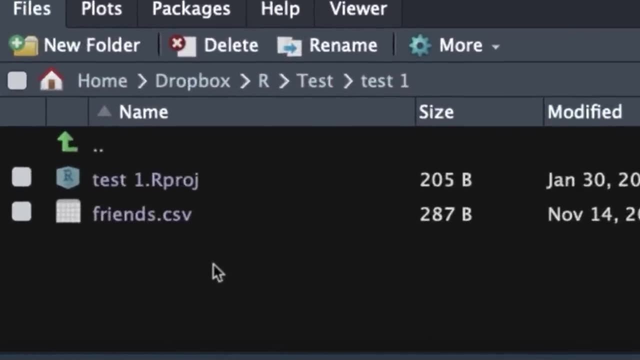 That's the folder that was created when we created our project. Go in there. I'm going to cut and paste some data into that folder. If we go back into R, we can see that data sitting here. Now that data hasn't been imported yet, We still need to do that. 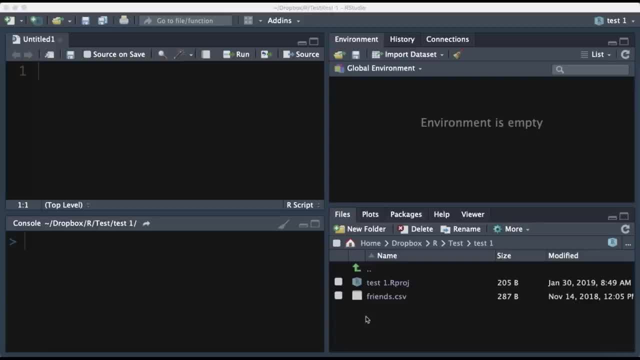 but at least we're going to be able to see it. So we're going to go back into R and we're going to click on import data set Now to bring that data into R, into our environment, make it into an object that we can use. there's a few things we can do And I'm going to show you the things. 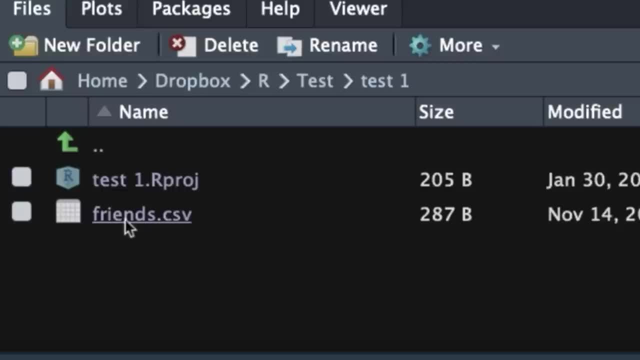 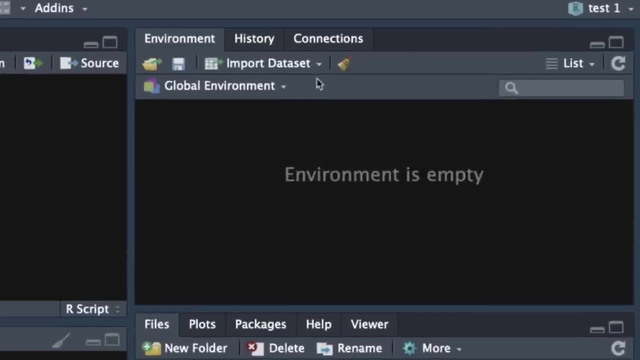 not to do, but just so that you know that they exist. If we clicked on this data down here, you've got the option of import data set. You can do that, That's fine. But I'm going to say: don't do that, There's other options. We've got import data set up here. Again, don't do that The best. 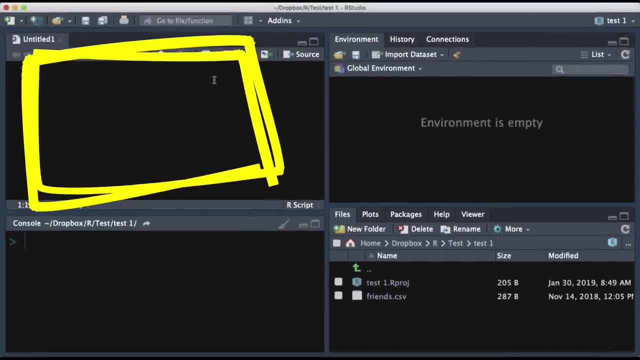 thing to do is to use your code, Get your actual script to go and fetch the data so that when you run your code it's automated, It automatically goes, fetches the data, creates an object, puts it in your environment, and you never have to think about it again. 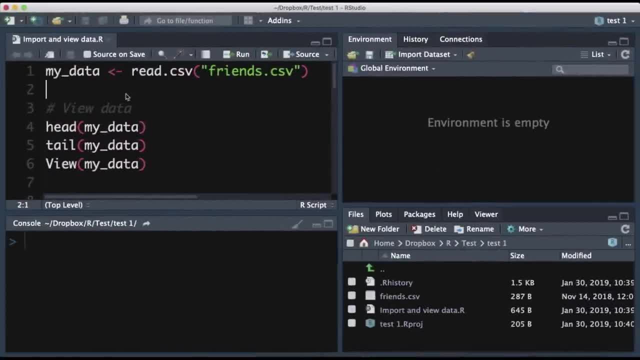 So that's the way to do it And I'm going to show you how, Right here, we've got some code, and this code is going to import some data And it's also going to do a little bit of analysis, And I'm going to go through the code one step at a time, just to teach you how it is that I've 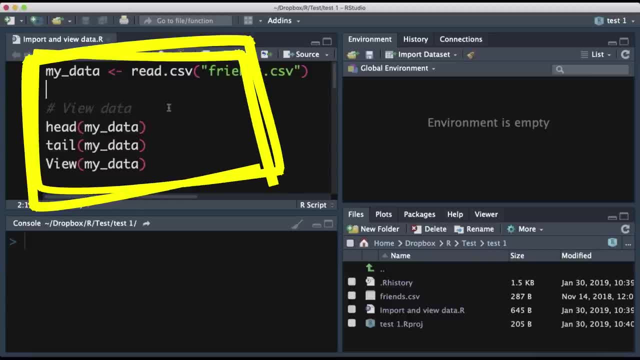 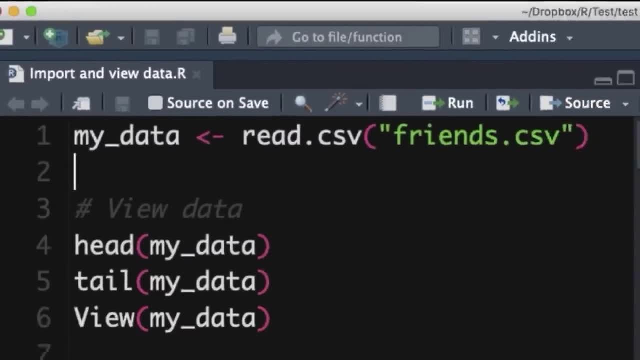 done this Right, Just so that you know when you write code here in the source up on the top left, if you, when you've written the code you put, go to file, save as, and you save it and it pops down here into your project which is all nicely and neatly kept in your 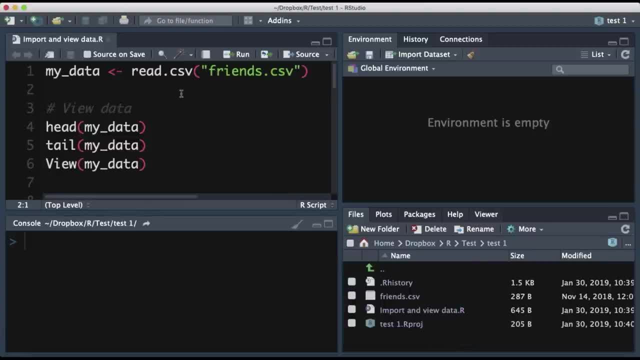 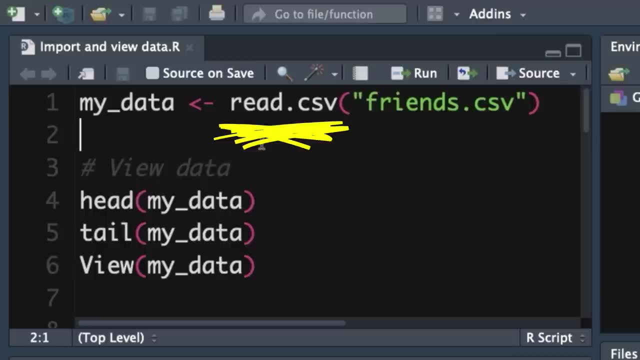 working directory down on the bottom right. Okay, So let's go through this one step at a time. Okay, We're going to start off by looking at the read CSV- read dot CSV- function. Of course, we can import any kind of data. We can import data straight from Microsoft Excel. 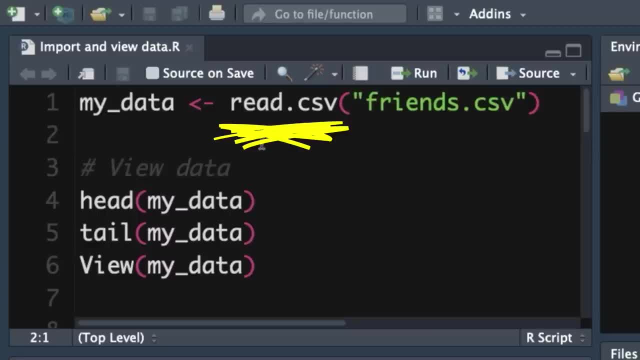 We can import SPSS files. We can import Stata files. A CSV is a nice and simple file. If you've got an Excel spreadsheet, you can save it as a CSV. I usually save files as CSVs and import them that way because it's uncomplicated and it's not messy. 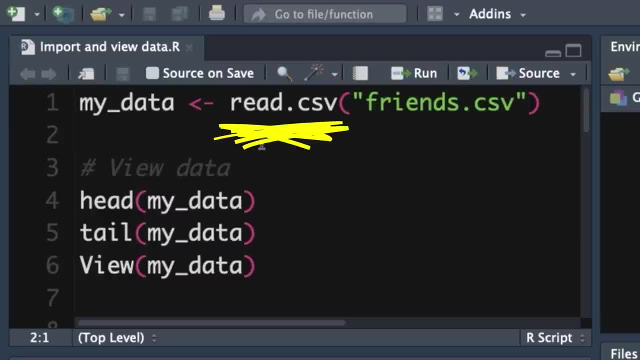 but we're going to create videos that look at each of these individually and, and, and we'll go through them one at a time. For this video, we're just going to stick with a nice simple CSV file. So we've got a function that says read CSV in brackets and in inverted commas. That's important. 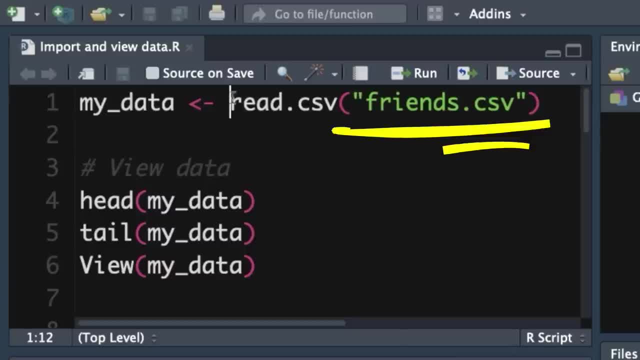 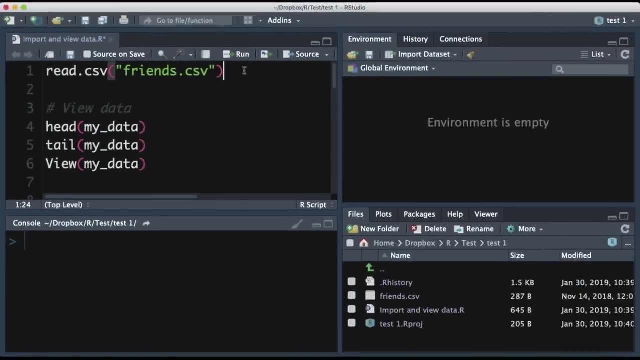 We have the file name and the file extension. Now, if I didn't have this little arrow over here, if I just did the function and the file, it's going to look in our working directory. I push command, enter to read the file. I'm going to look at the file name and the file extension. 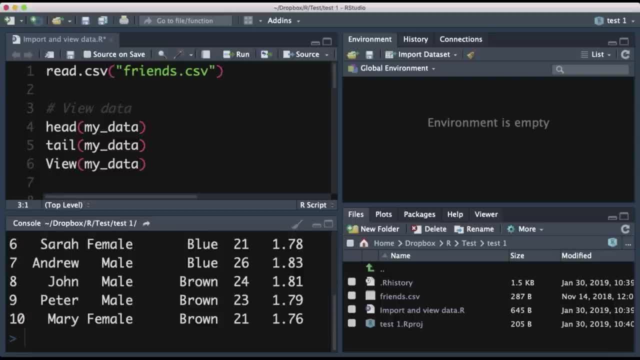 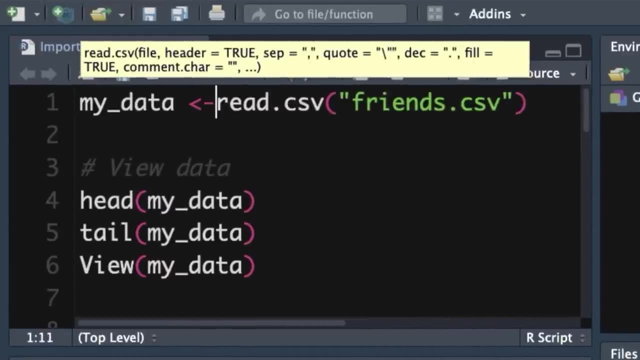 Run that or I click on run over there, So command, enter and down here in the console we can see there's our data. Now that's not particularly useful to us right now, as it is because we want that to be an object that we can use. So if I give that a name and I say my data and create this, 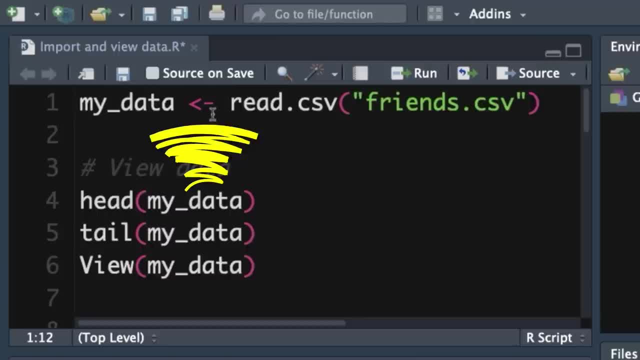 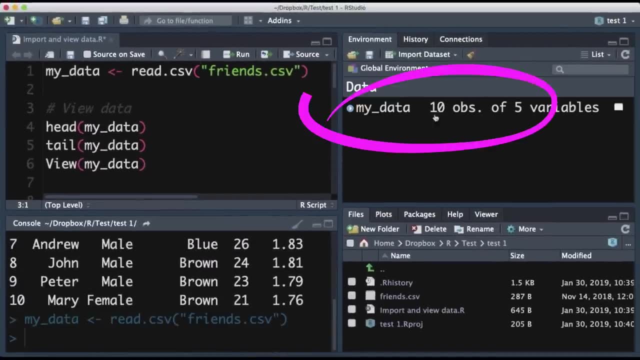 little arrow with the less than and dash, which is kind of like an arrow. it says everything that's over here gets assigned to that name: push, control, enter And in our environment on the left we can see my data sits there. We can have a look at what the variables within that are And that's our. 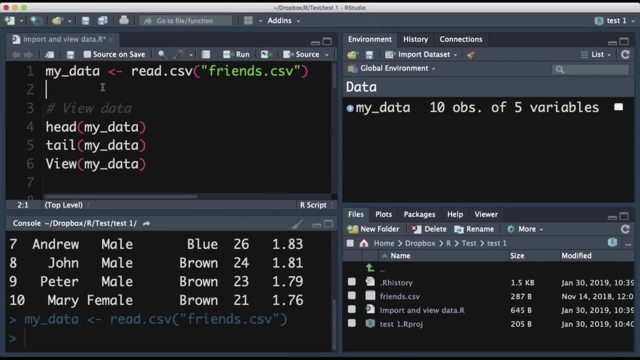 data sitting and it's been read in and it's within R and we can start using it. So we want to view our data Now. for the most part, R works with functions and objects. So we've got an object- my data- sitting in our environment over there and we've got functions. A function is this function? 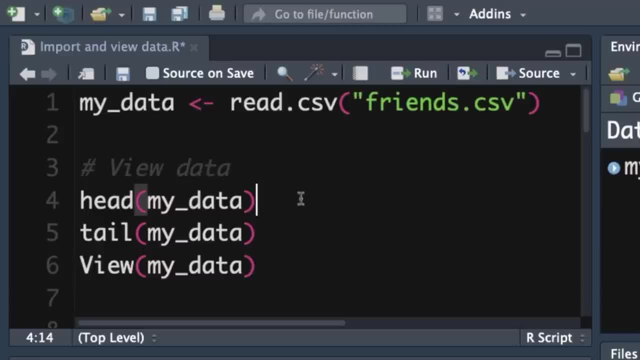 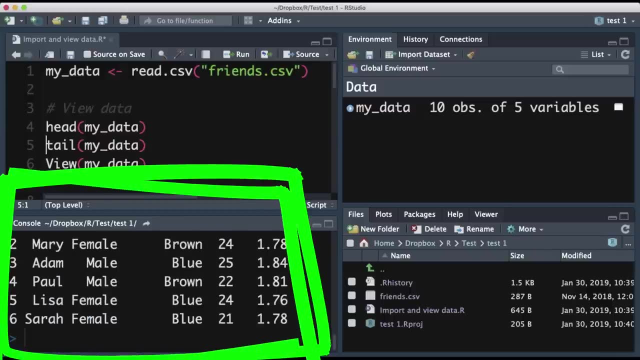 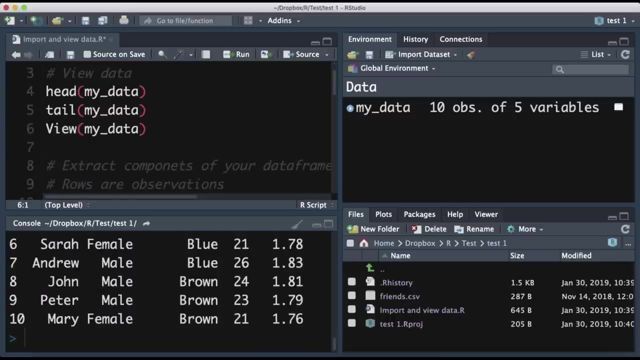 called head. If we type in head my data and push command, enter or control, enter or run up there it's going to give us the first six rows of data. If we do tail my data, it's going to give us the last six rows of our data. And if we do view my data, it's going to produce the data in a little. 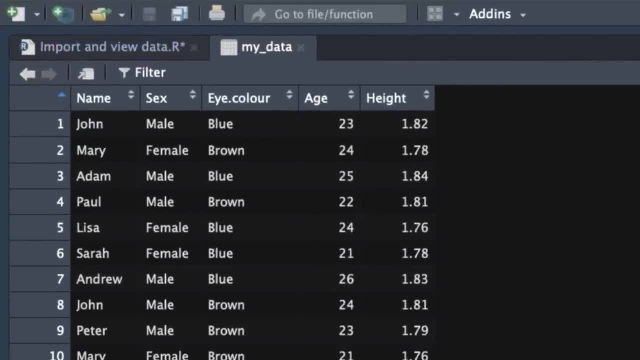 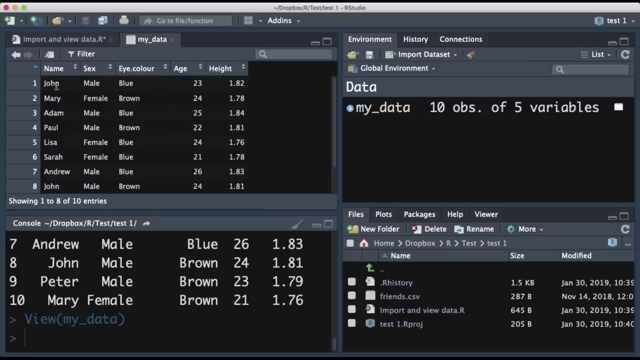 spreadsheet that we can look at. So let's have a look at that Right. Remember, with this kind of data, this is a nice flat spreadsheet We've got. each row is an observation and each column is a variable. Let's go back to our four quadrants. We can also view the data If we 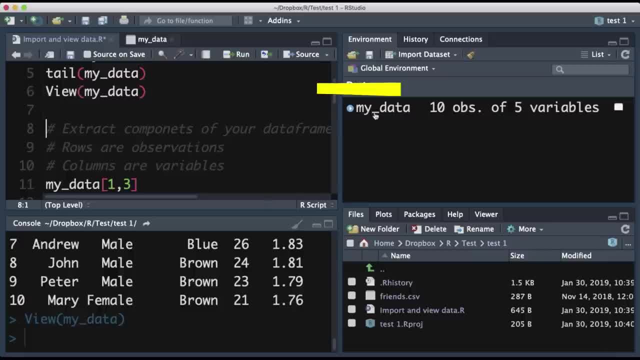 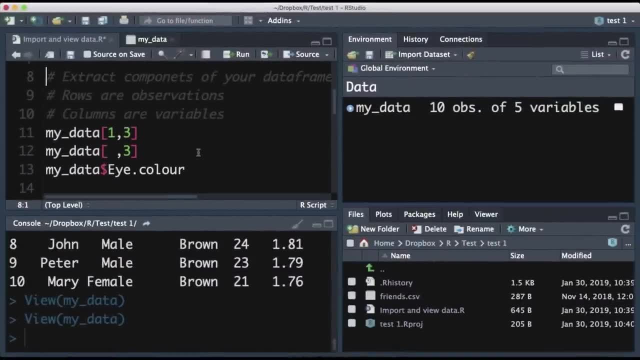 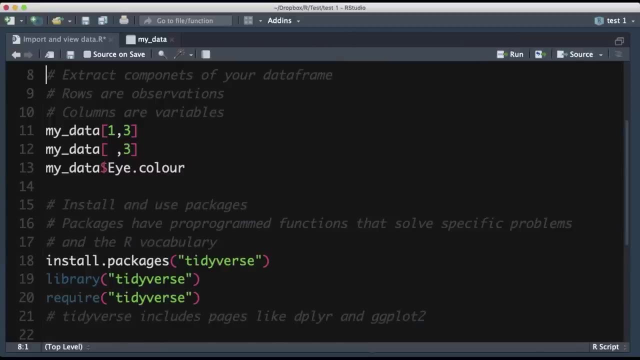 look at our script. we can also view the data by clicking on my data. We can click on the object and it'll also bring it up over there. Now we might want to extract specific components of our data. So remember we've said that rows are observation, columns are variables, And if we 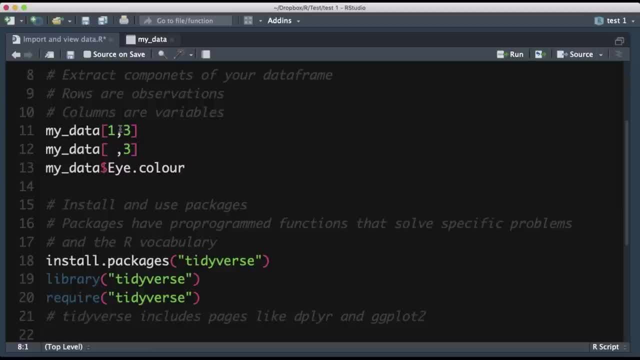 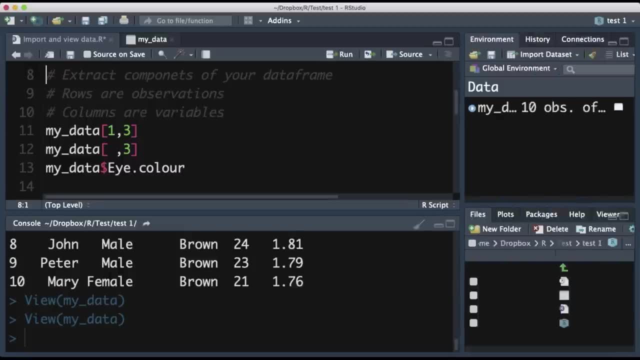 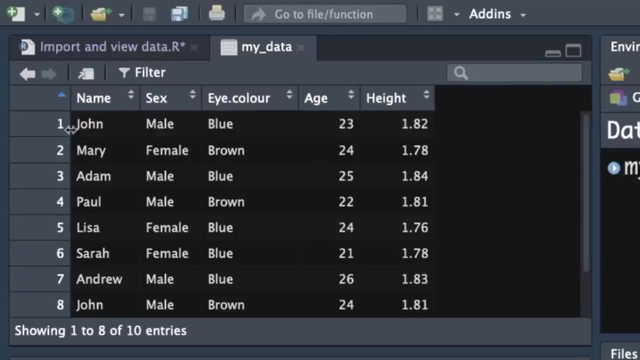 put my data and we use these square brackets to tell R where to look. the first number after the square bracket tells it what row to look at and the second number what column, Right? So if we run that, it's going to give us blue. Well, what is blue? Blue is the first row. 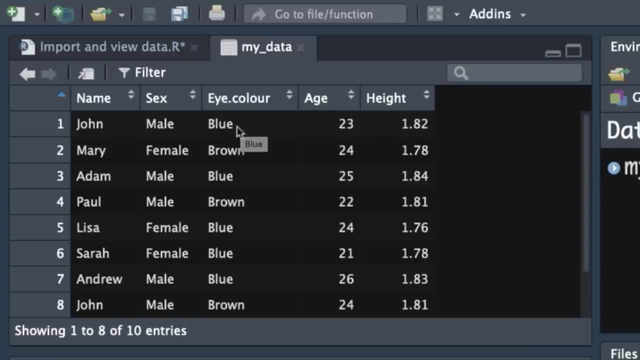 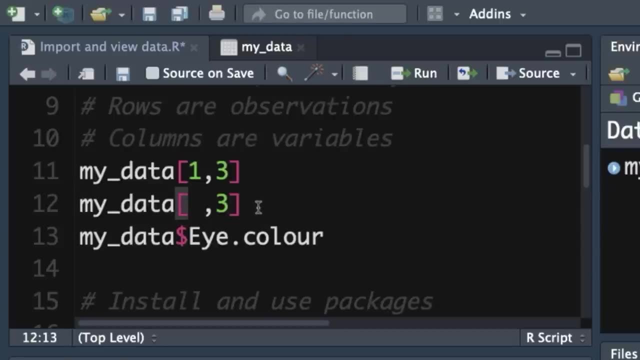 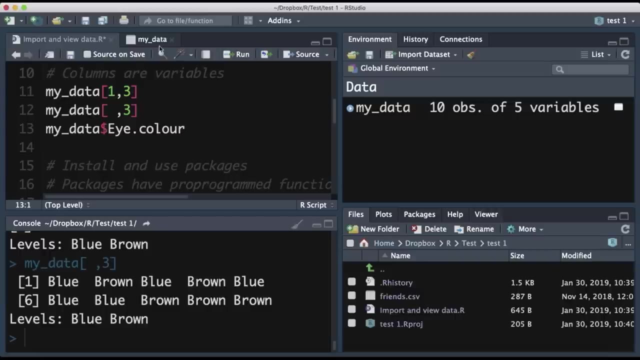 and the third column, the variable iColor. So we've got this cell over here popped out. If we didn't put a row and we just put comma three, it's going to do the entire column. So let's run that And there we go: Blue brown, blue brown, blah, blah, blah, blah. That's. 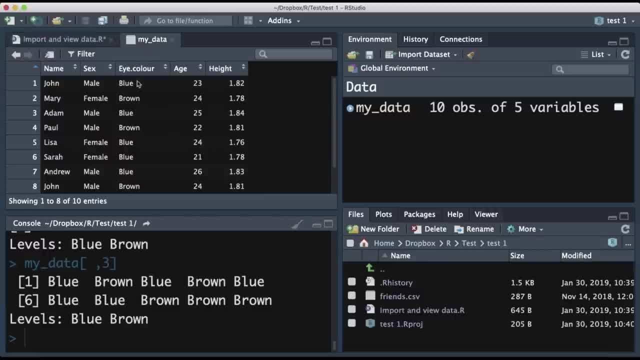 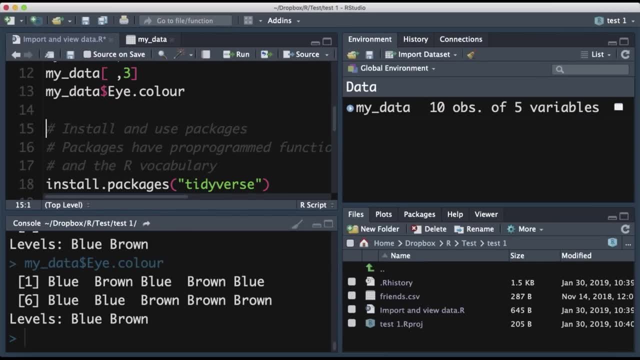 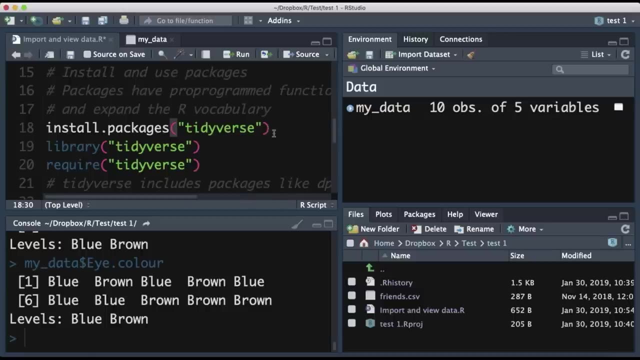 basically spitting out this entire column And this column. this variable name is eye color, so we can also do my data, dollar sign, eye color- and it does the same thing. okay, before we start doing some analysis, I just want to talk to you a little bit about packages, because you're going to find these things tremendously useful, right packages? 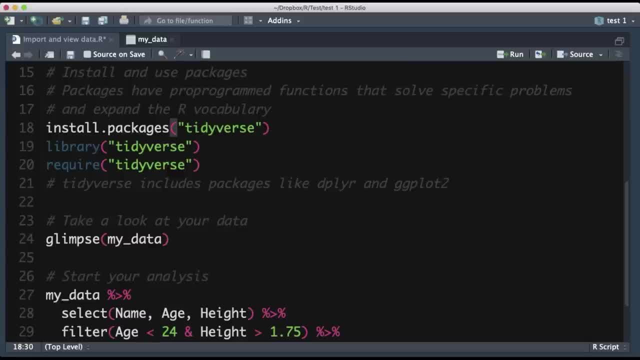 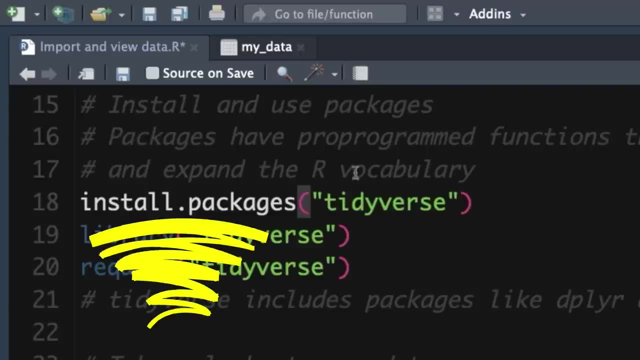 are pre-programmed functions that solve very specific problems. they expand their vocabulary. to install a package. you use this function: install packages right and then open brackets. you need the inverted commas. you put the name of the package. close brackets. you only ever need to install a package once. once it's installed on your computer, it's there, but when you want to use it in your 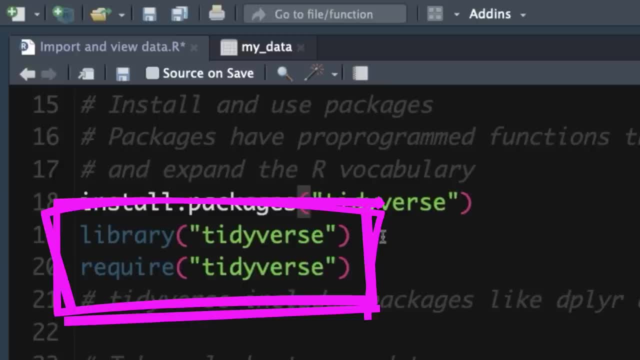 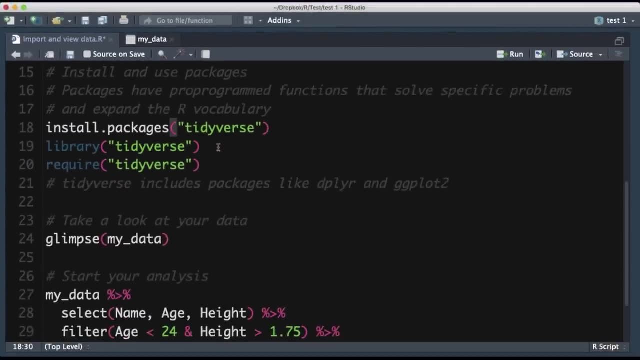 script. you need to include either library or require either of those two. you don't need them both. you put that into a script, it'll go and fetch that package, it'll use it and then from that point onwards in your script you have access to additional commands and functions. so of course, 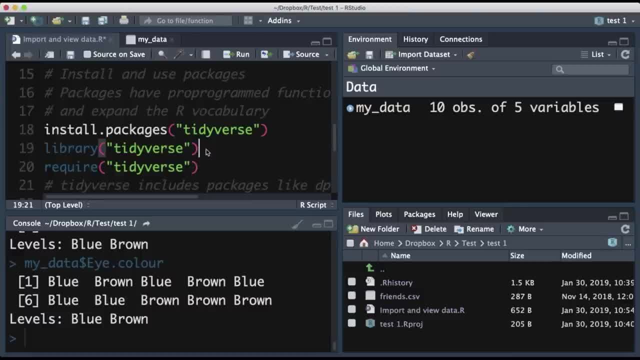 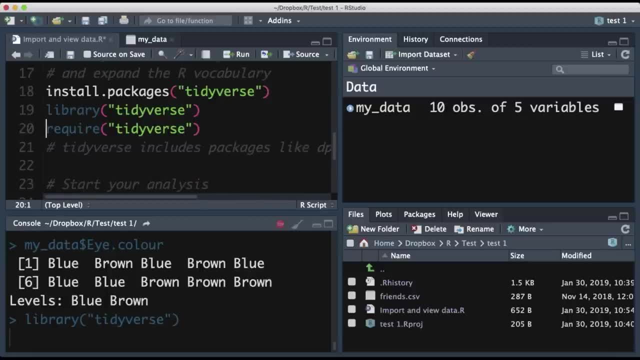 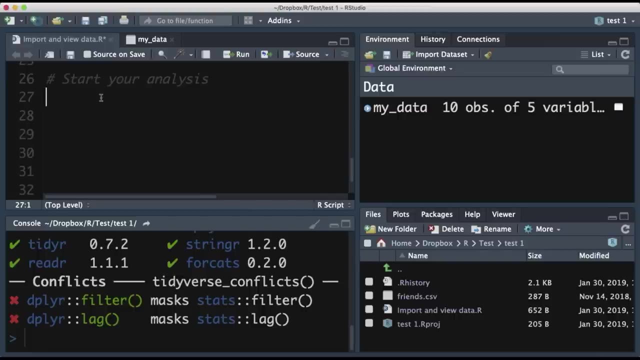 I have previously installed the tidyverse package. at this point I want to push command enter or control enter to run this line of code that uses it so bada bing. now I'm going to show you how to do an analysis in our using some of this vocabulary that comes with the tidyverse. 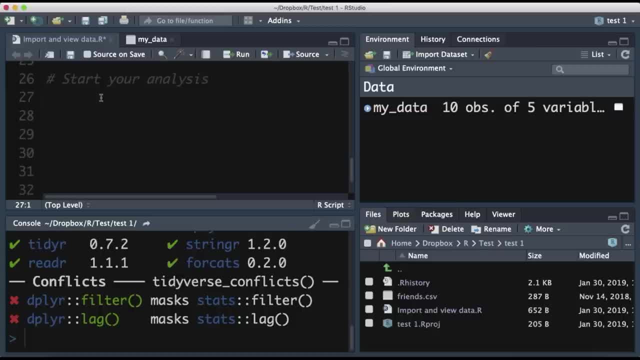 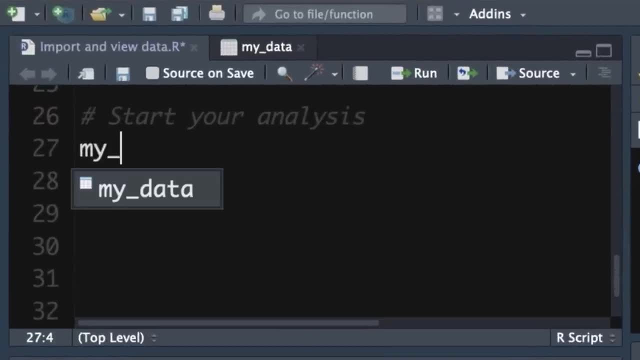 you're going to see how easy and intuitive and straightforward it is, and when you see how easy it is, you're going to be really excited about analyzing your own data. okay, so the first thing we do is we type in our data frame. we start off with my, my data, that's our, that's our object. okay, 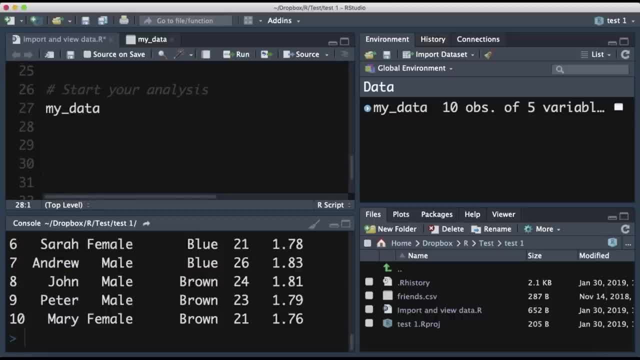 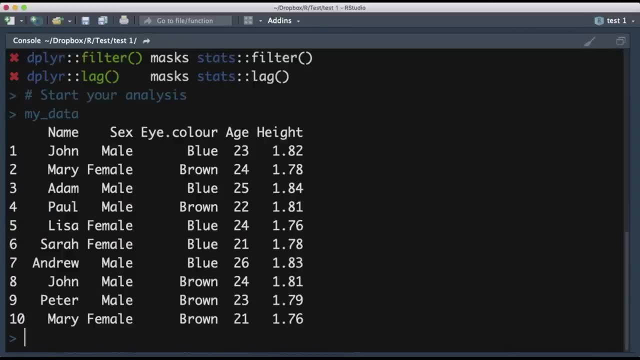 well, I'm going to actually press on it. I'm going to go to the door and I'm going to say, oh my gosh, yes, here we go. ok, let me press on the door and my data is el prolongated and I'm going to to normalize that data frame. we're so you've got the data frame. 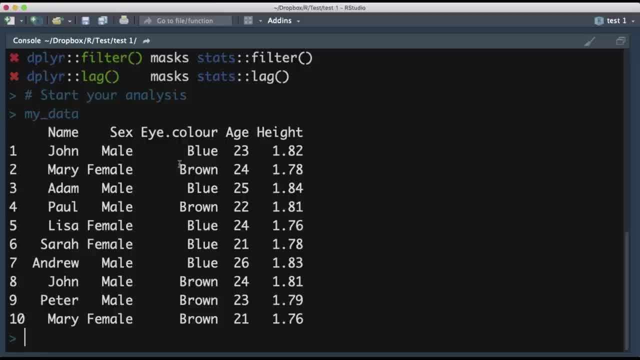 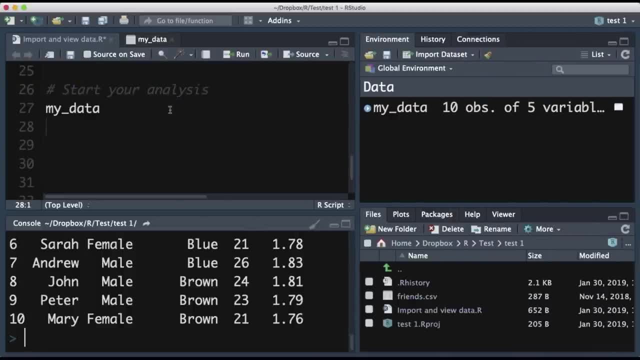 the size of it you get. the bit can be a bit longer, it can be bigger, even a bit bigger, And we might in this case want to select just name, age and height. right Shift-Ctrl-0 to go back to all four quadrants. 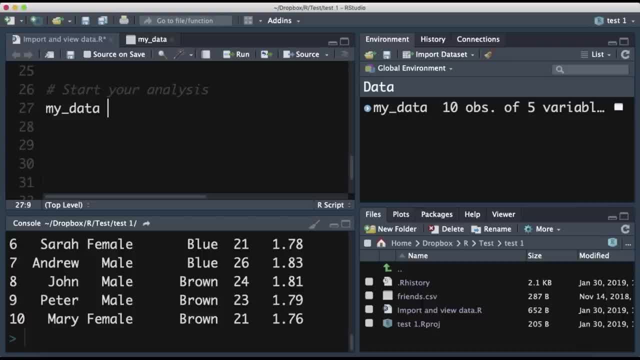 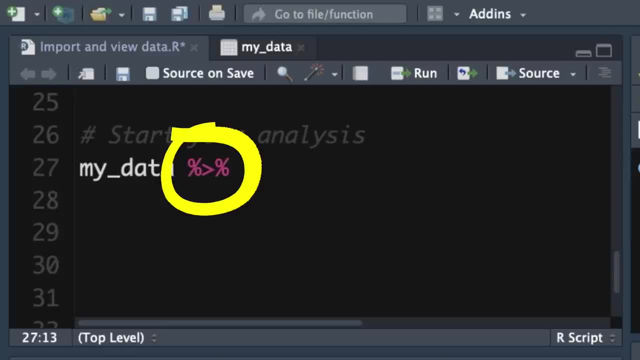 So we want to select that. Before we select it, I want to teach you about a little thing called the pipe operator right- Shift-Command-M. That's the pipe operator right. It's a percent greater than percent. It looks a little bit like a pipe. 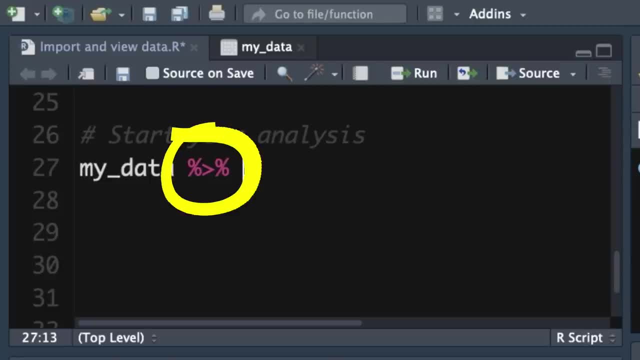 And what it means is whatever you've done on the left-hand side, whatever that line of code is, gets piped into the next line of code, right? So if you've done some sort of change or manipulation, that change gets piped into. 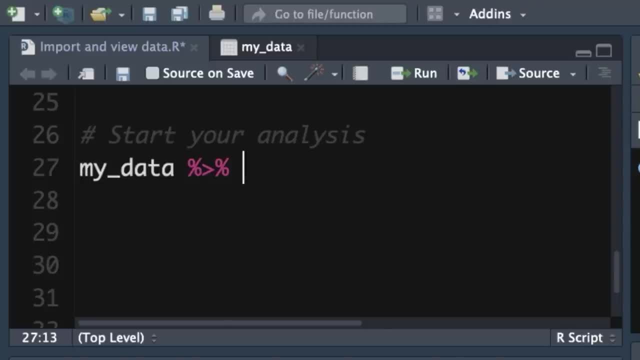 And you'll see more how that works as we go through this example. Now you could just carry on typing to the right. I like to, after a pipe operator, go to the next line. R will see that as continuing on the same line. 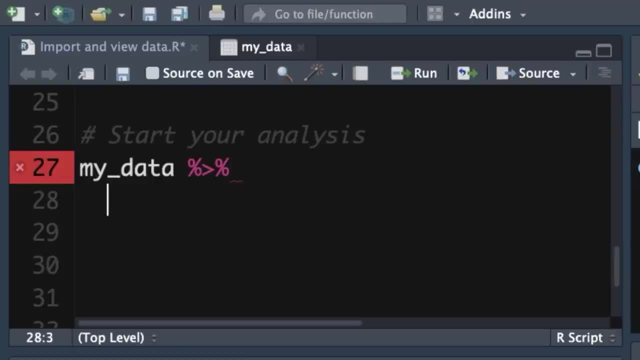 It doesn't really matter. Okay, it looks like an error is popping up there. It's not, You can ignore that red. Okay, so we've said my data We've got in a pipe operator, which just means and then 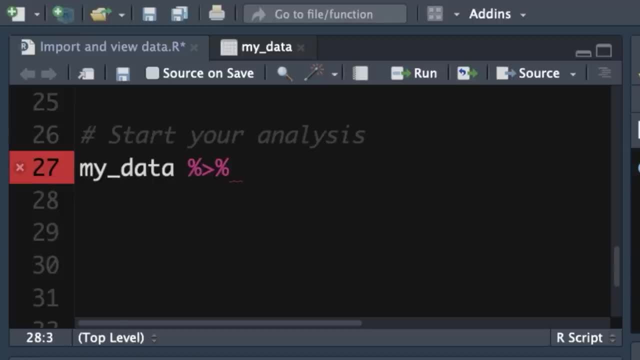 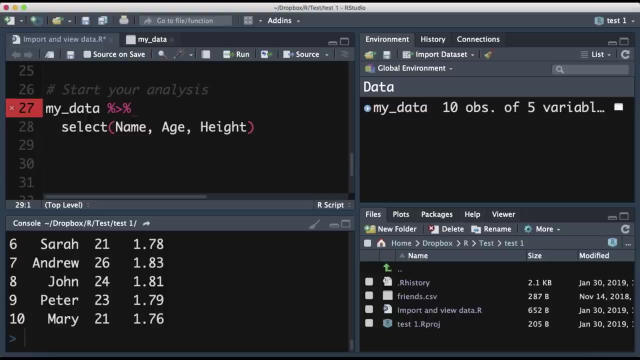 So my data. and then right, We've said we want to select name, A, H and height. So it is literally as simple as that: Select open brackets, name, age, height, command enter. Okay, Now we can see in our console and I'm going to zoom in on the console with shift control. two: 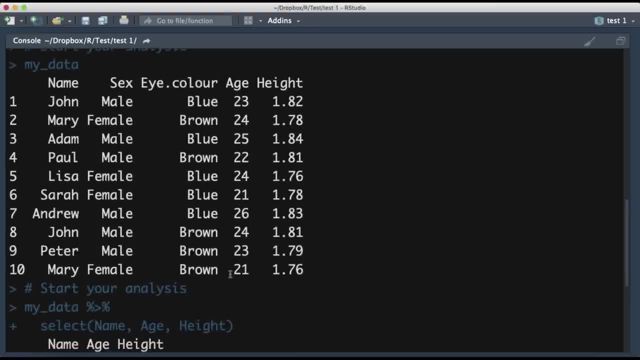 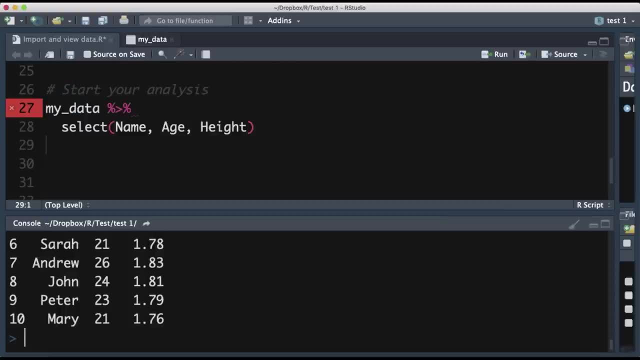 We can see. we originally had the entire data frame. We wanted to select a few of the variables, in this case name, age and height, And there they are. Now we might want to only look at people, People that are less than 24 years old. 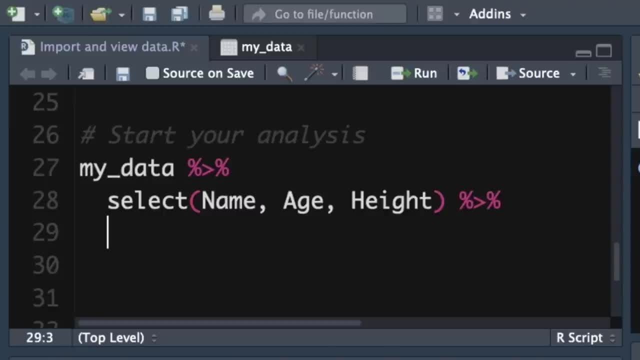 So another pipe operator which is, and then Go to the next line Filter by those that are aged less than 24.. And we might want to say: let's make this a bit more complicated and say age less than 24.. And height greater than 1.78..